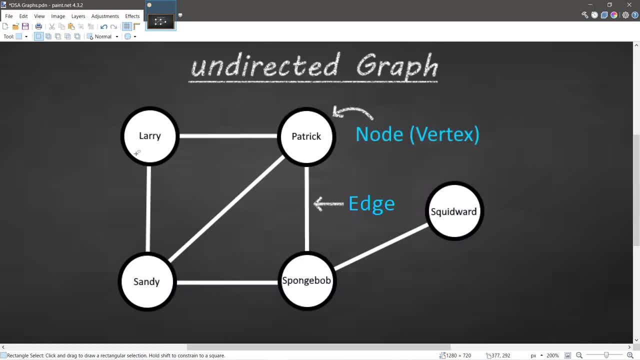 what is known as adjacency. In this example, Larry is friends with Patrick and Sandy, so Larry has adjacency to Patrick and Sandy. Patrick is friends with Larry, Sandy, SpongeBob and SpongeBob is friends with Sandy. Patrick and Squidward and Squidward is adjacent to only one neighbor. 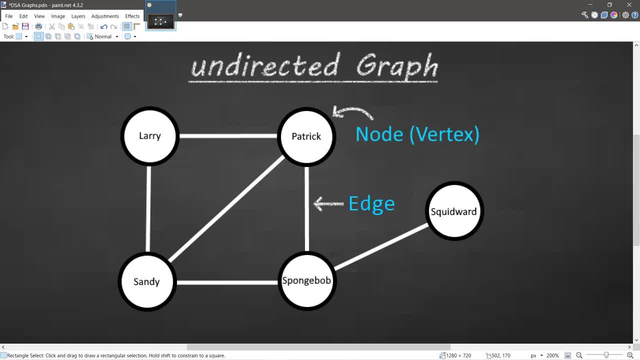 SpongeBob, SpongeBob, So a social network could be an example of an undirected graph. The other type of graph is a directed graph. A directed graph contains edges that will link one node to another. However, these are one-way connections. In this example, node A would have adjacency to node B, but not. 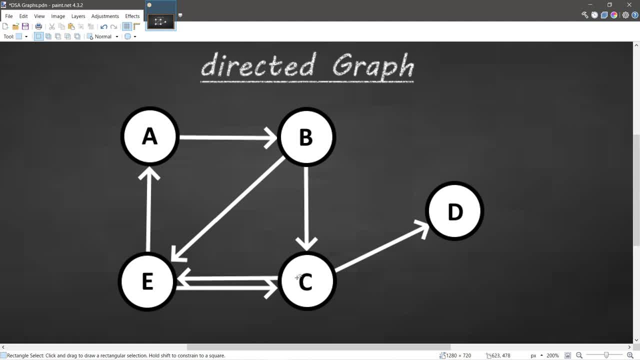 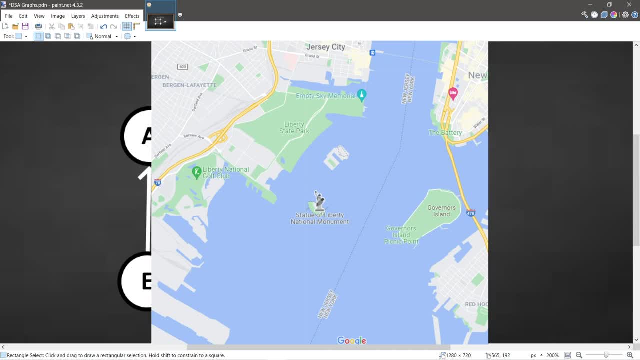 the other way around, However. it is valid to have one node pointing to another node and that node could point back to the previous node. An example of a directed graph could be a street map. Let's say: you're working on a street map and you're working on a street map. You're working on a. 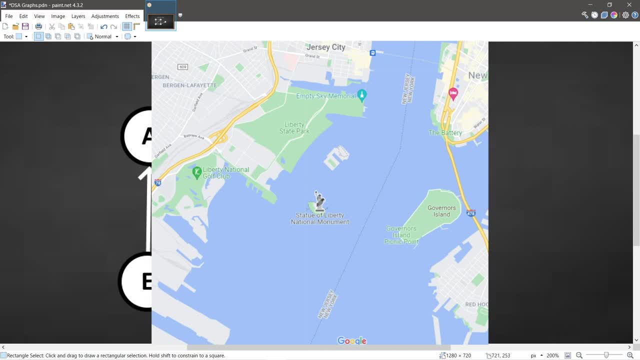 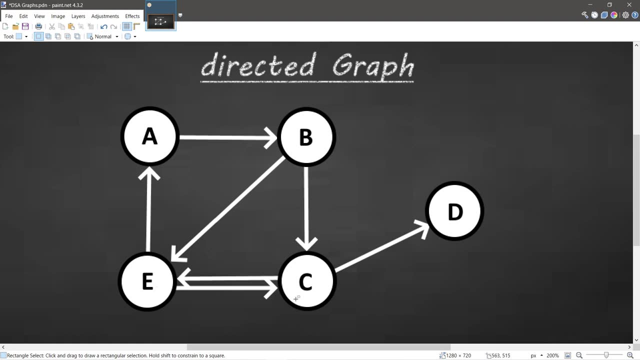 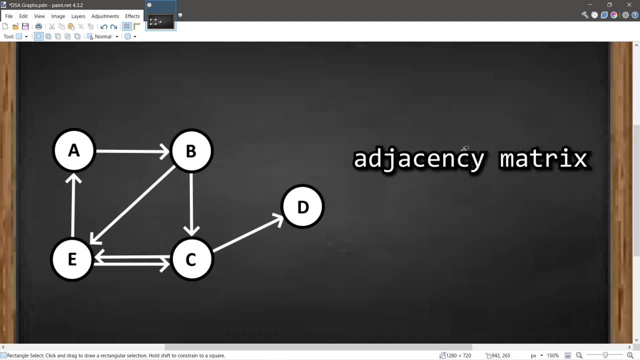 travel app and each node is a possible destination. These single edges could be one-way streets and these double edges could be two-way streets. You can move back and forth between these two destinations. There are two popular ways to represent a graph: an adjacency matrix and an 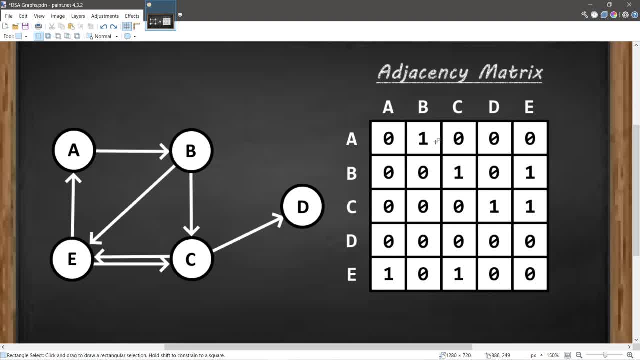 adjacency list. With an adjacency matrix we could create a 2D array, one row and one column for each node. If we need to check to see if there's adjacency between two nodes, we would first find the index of the node we're beginning at, let's say A. So we would go to node A. 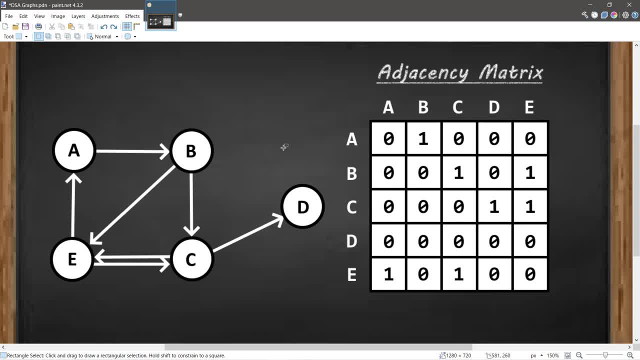 and then find the index of the node we're trying to travel to. so B. So row A, column B: If there are no edges, this would be zero. If there is an edge, this would be one. So, since there's one here, 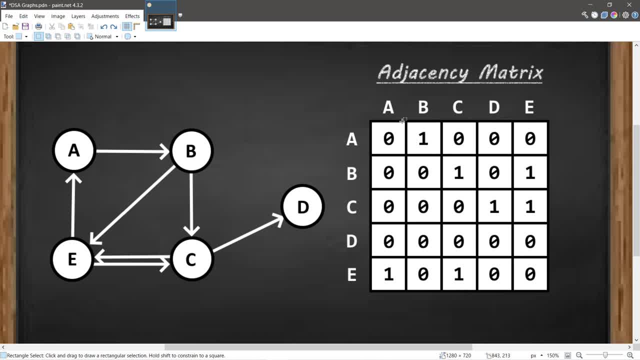 within row A, column B. well, there's adjacency from node A to node B, But if we take a look at row A, column C, this is zero. so there's no adjacency between A to C. But if there was, well, we would replace the zero with one. then Now there are pros and cons with the matrix. 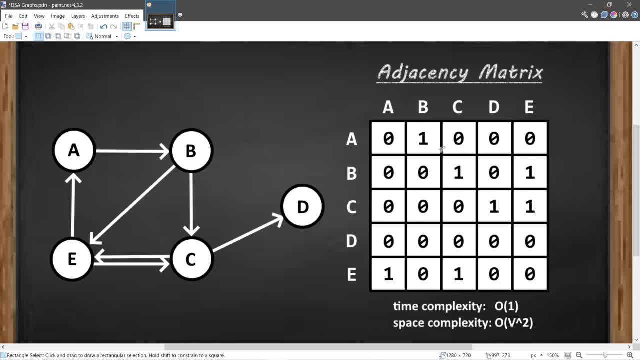 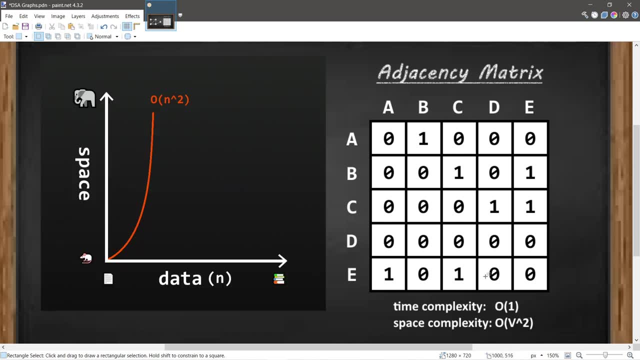 One of the benefits is that the runtime complexity to locate an edge is O. it's constant. All we have to do is find two indices, So we have to find the row and the column. However, the space complexity to store a matrix is O squared V, as in the number of vertices that 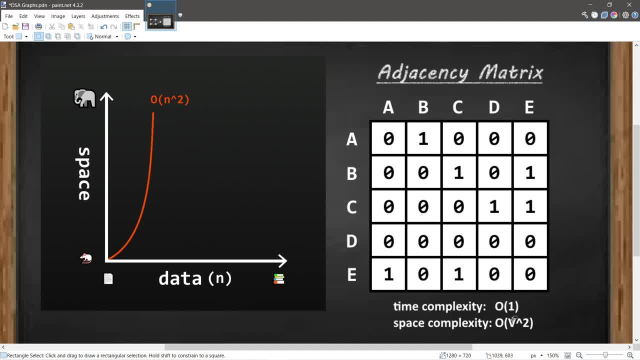 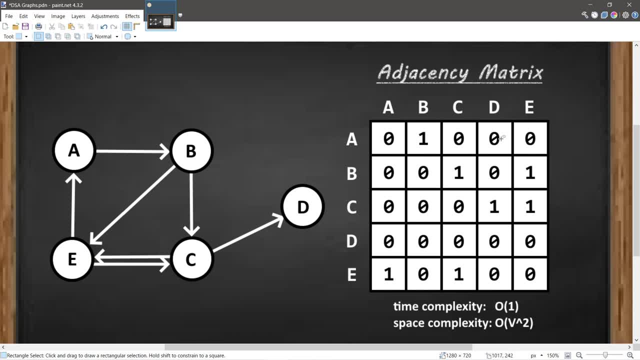 we have. But you could also think of that as N, N for the number of nodes, O. So since we have five nodes and five columns, we would have a total of 25 spaces. So the benefits of a matrix is that it's very quick to look up an edge. However, a matrix uses a lot of room, So it 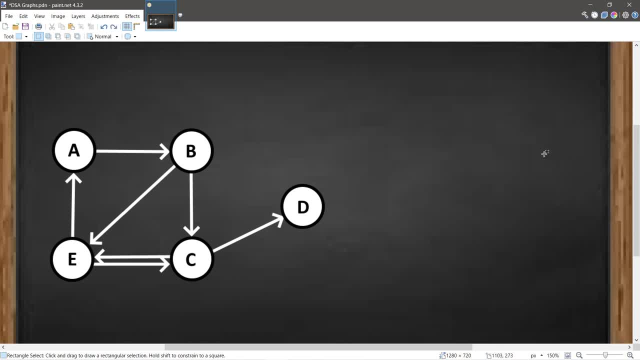 tends to suit graphs that have a lot of edges. On the other hand, we have an adjacency list. An adjacency list is an array or array list of linked lists. Each element is a separate linked list And each header within the linked list would contain the 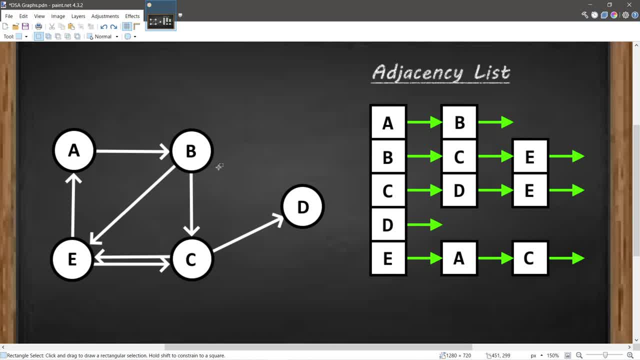 address of a node. If there's adjacency between one node and another, we would add the adjacent node to our linked list. So to find adjacency between two nodes, we would find the node that we're starting at. Let's see if B is adjacent to E. So we would locate index B and travel this. 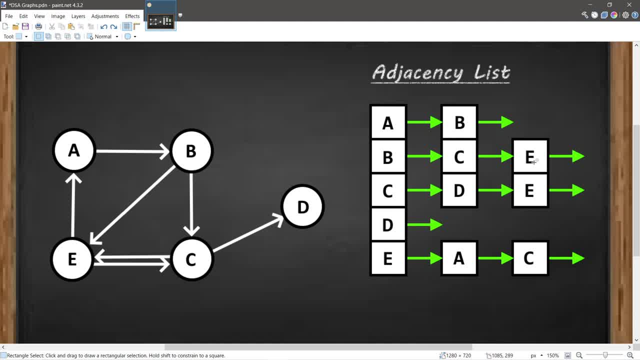 linked list until we find the node that we're looking for. That means there is adjacency between nodes B and E. Even if there's a node that is not adjacent to any neighbors, we would still want to add it to our adjacency list, Just in case. 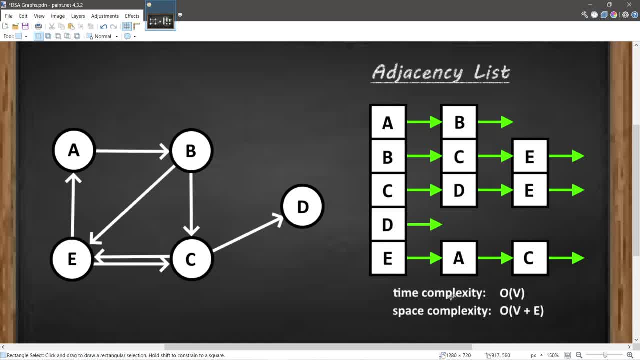 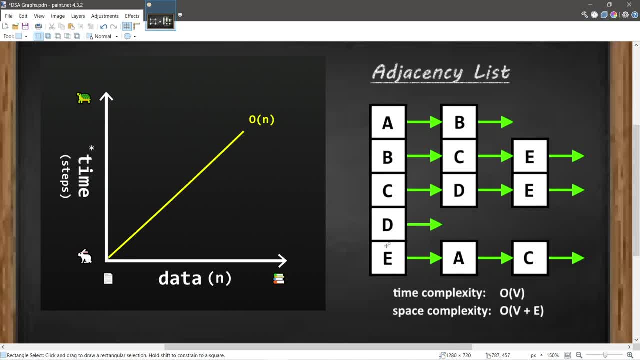 do update it. Here are the pros and cons of an adjacency list. The time complexity to locate an element is big O of V, V, as in the number of vertices You can also think of this as N, So this would be big O of N. To locate an edge, we would first access the node that we're beginning. 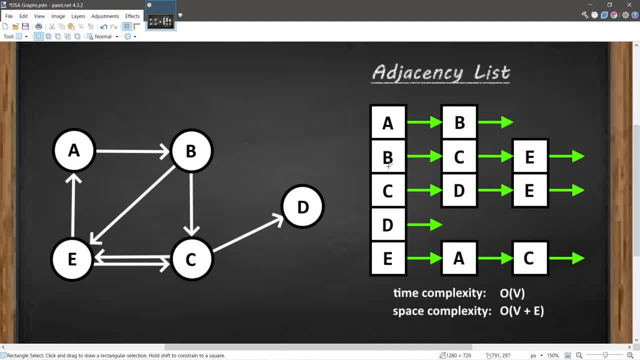 at by an index. So let's begin at B, and we are looking for adjacency between B and E. Since each element is a linked list, we need to traverse this linked list linearly until we find the node that we're looking for. So in that way it's linear. However, a benefit of a list over a matrix is that 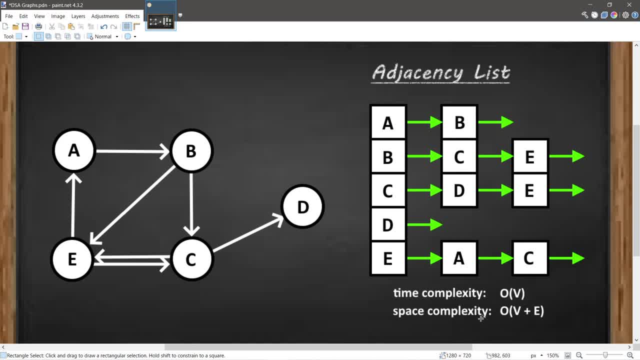 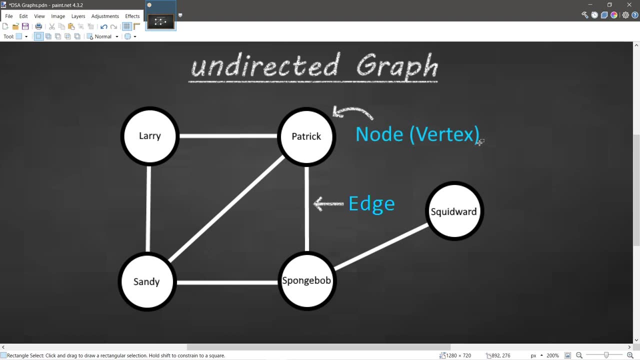 they use less space. The space complexity of an adjacency list is big O of V plus E, V for the number of vertices, aka nodes, and E for the number of edges. So yeah, everybody, those are graphs. A graph can be used to model a network. Each node is a piece of data within our network and an edge. 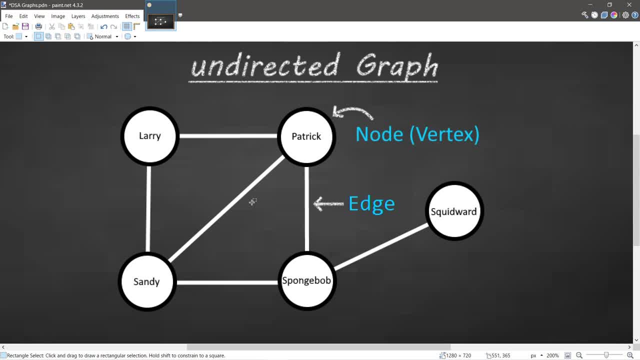 connects nodes. So, like I said, it's a popular way to model a network. Each node is a piece of data within our network and an edge connects nodes Which don't necessarily have any sort of order. So yeah, that's an intro to graphs, and in the next,